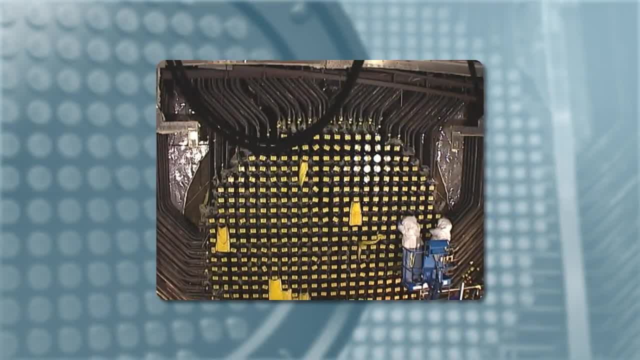 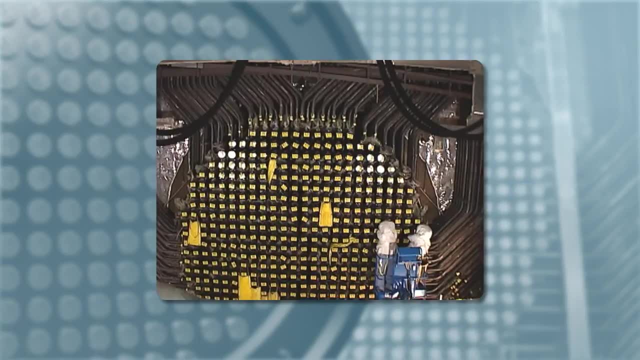 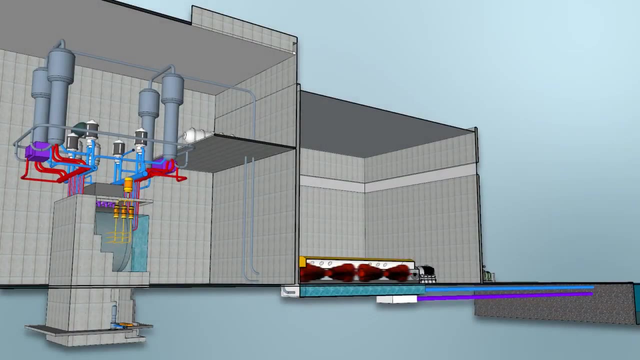 Pipes and other components are maintained and inspected regularly and replaced if needed. Inspections include measuring pipe wear and tear And identifying any microscopic cracks or changes well before they become a problem. The second system, the steam system, uses normal water. The heat from the reactor turns 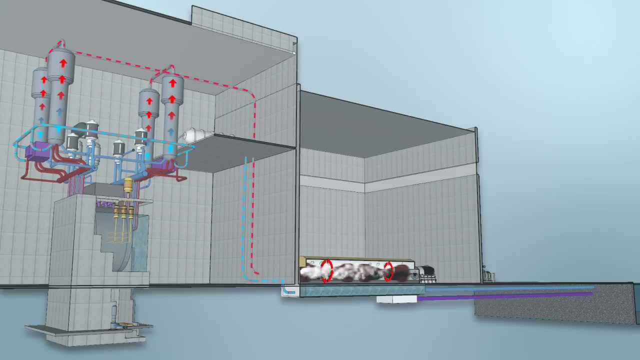 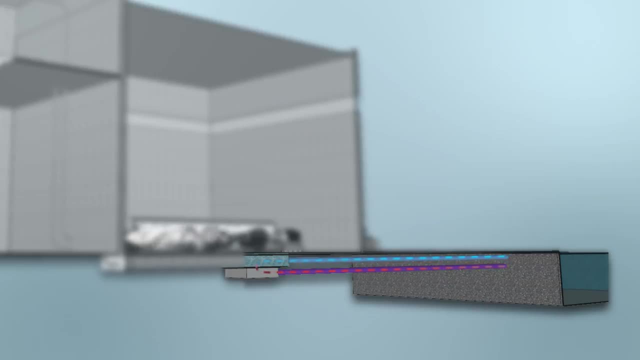 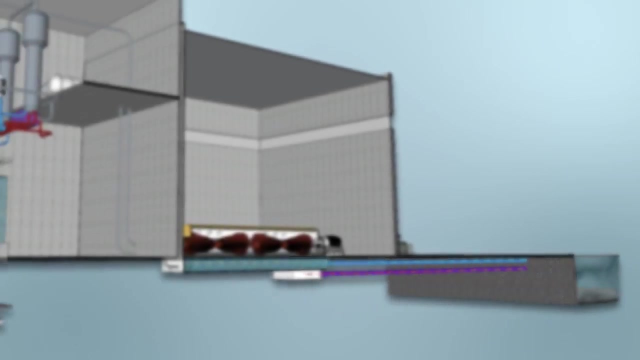 this water into steam to run the turbines and generators. That steam is then cooled and condensed using a third system that pumps in cold water from a body of water such as a lake or reservoir. This is called the condenser cooling system. Like other components, the steam and condenser cooling systems are regularly inspected. 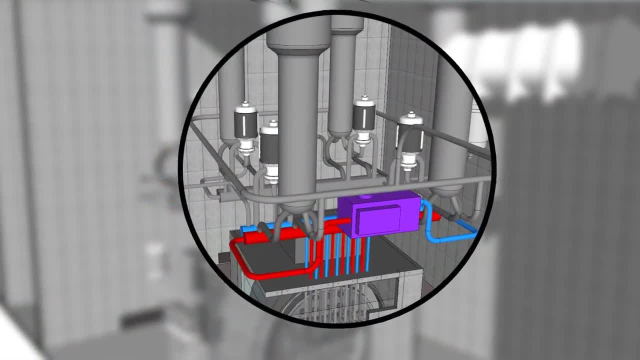 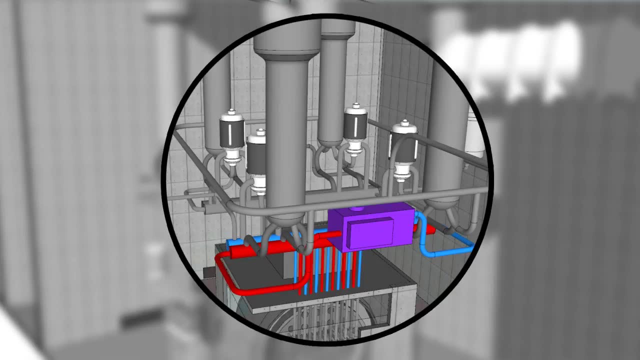 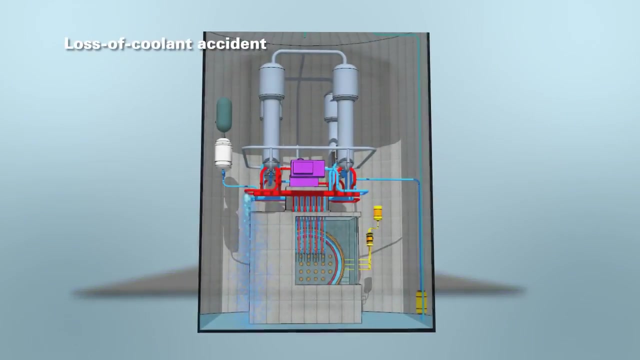 A simpler cooling system is used when the reactor is shut down for an extended period, for example during a planned outage. It requires little power to function and is connected directly to the heat transport system In the unlikely event of a loss of heavy water. 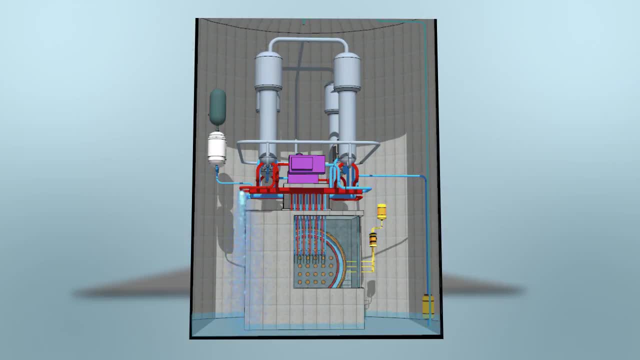 which could, for example, be caused by a pipe break. emergency injection systems would ensure water continues to circulate over the fuel to cool it. Emergency injection systems would work with pressurized tanks of nitrogen or pumps. All plants have two or three injection systems, A collection basin located in the basement. 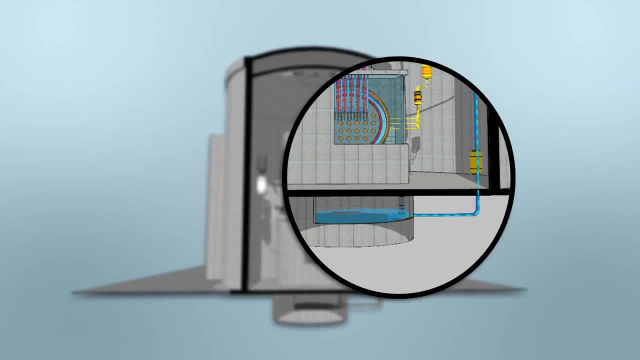 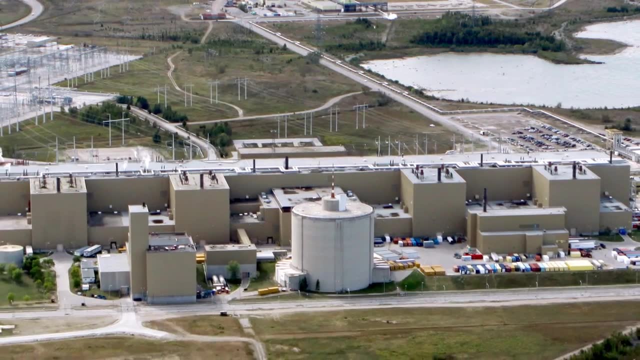 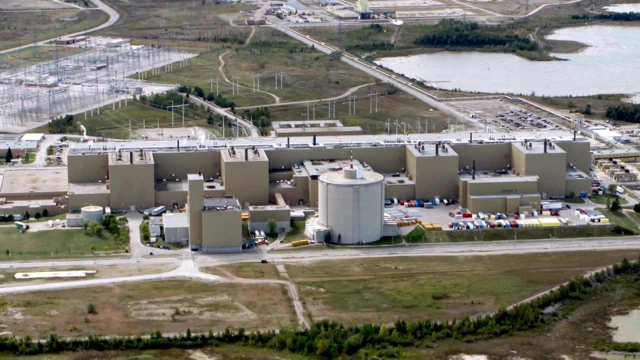 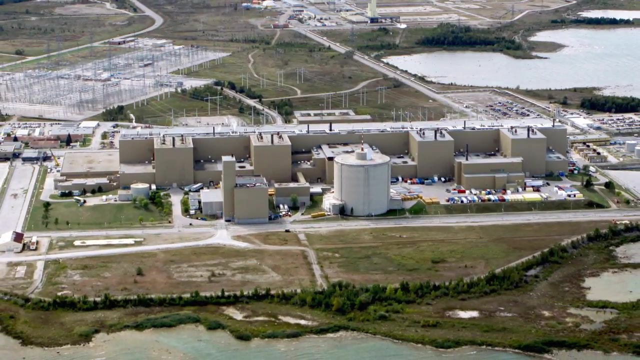 of the reactor building would recover the water and pump it back into the reactor until repairs are made. Electricity is needed for all cooling systems to operate normally. Nuclear power plants in Canada are equipped with multiple sources of backup power if they get disconnected from the grid. Sources of backup power include on-site power, that is, the power produced by the plant. 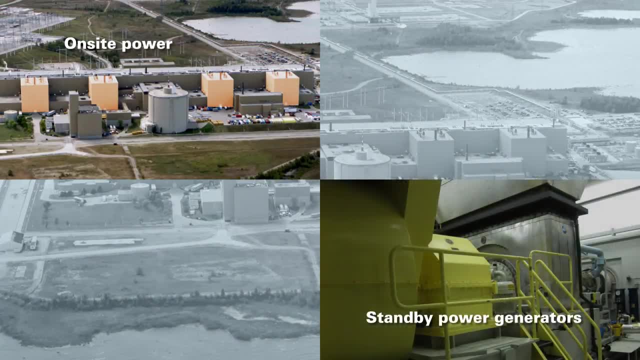 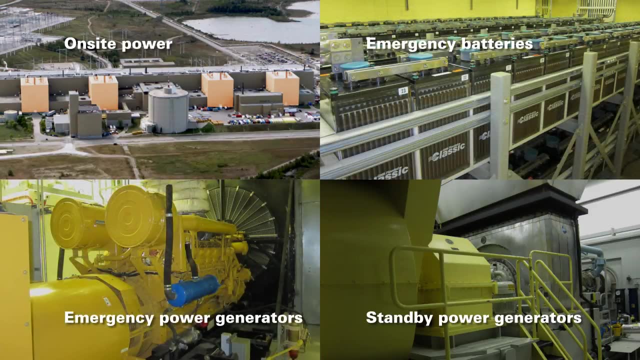 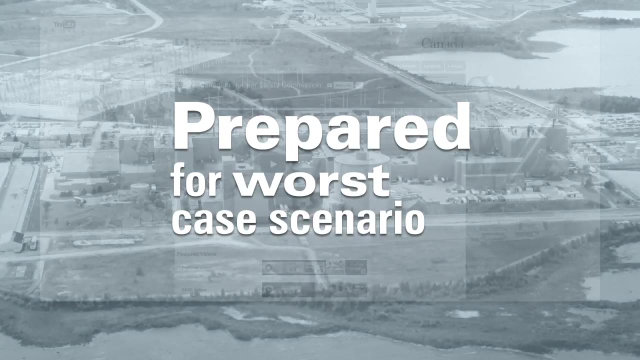 itself. In addition, at least two or three standby power generators, two or three emergency power generators and emergency batteries are available. You can learn more by watching our video that describes what would happen in the very unlikely event of a total station blackout.